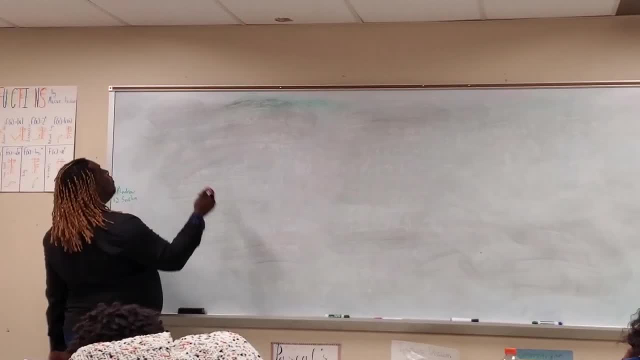 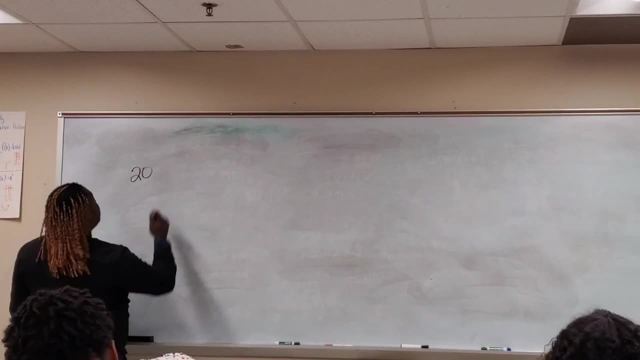 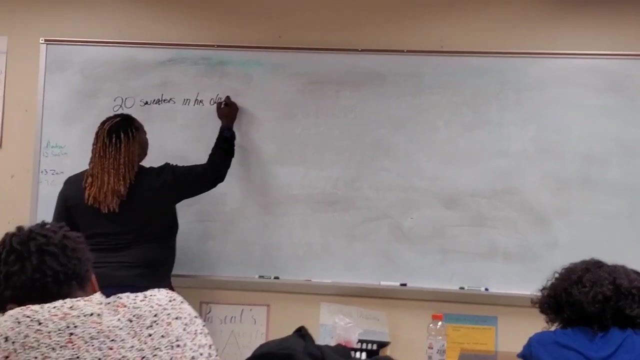 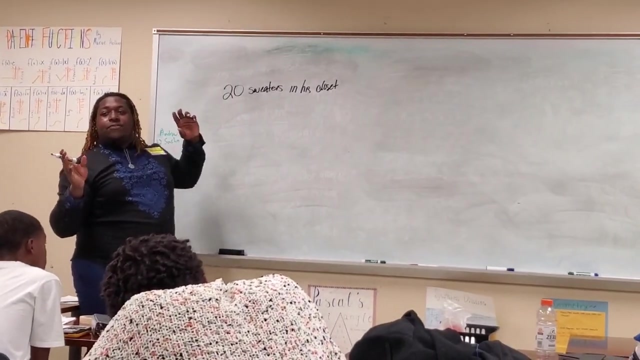 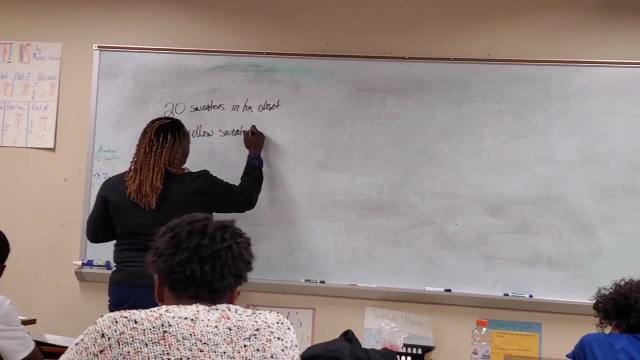 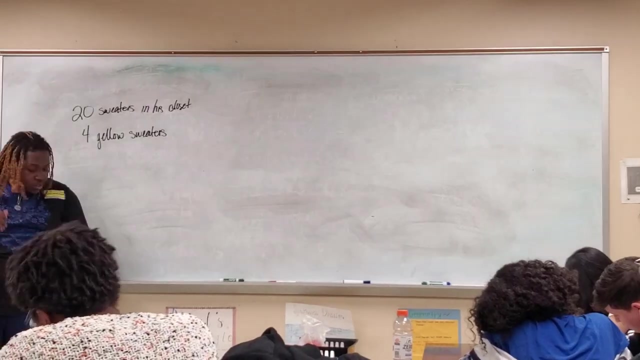 Let's say that he has 20 sweaters. Let's say he has 20 sweaters in his closet, But of the 20 sweaters that he has in his closet he has four yellow sweaters. So if Mr McDonough is getting dressed this morning, he's standing in front of his closet and he's like I don't know which sweater I want to wear today. 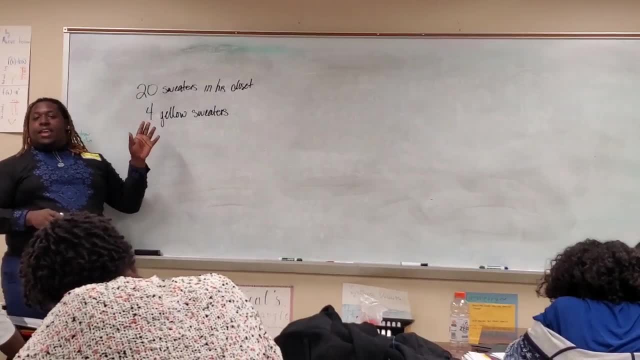 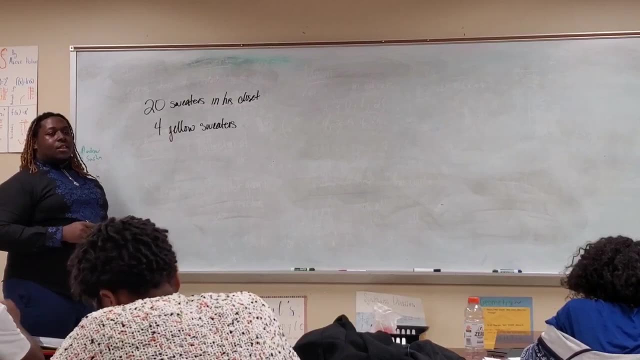 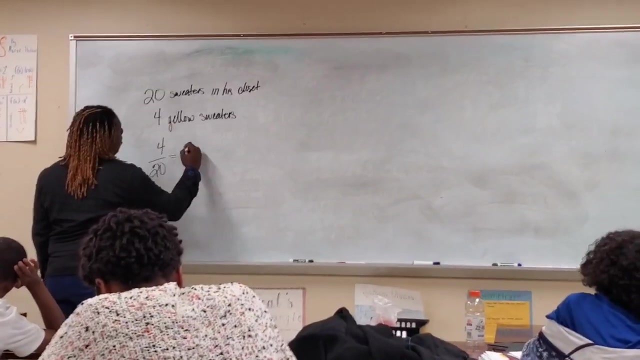 What is the probability that he decided to wear a yellow sweater? Yes, How did you get one-fifth? Because it's like a fraction, so it's more than 20 sweaters are yellow, So we just need to simplify that fraction. 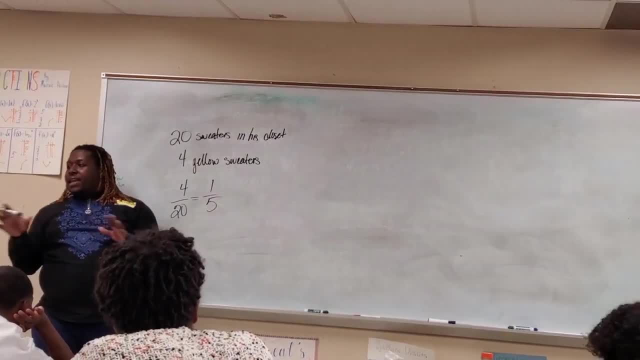 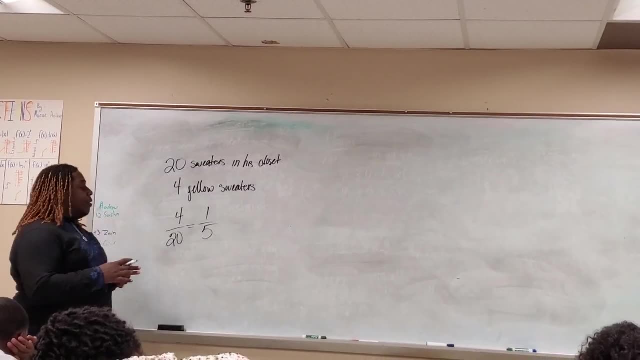 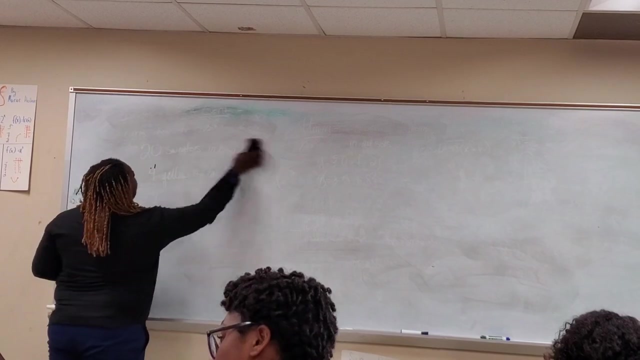 Here we go. When it comes to basic probability, it's just fractions, And y'all worked with fractions before, so I know that's not new. So that's all. basic probability is. Now we have this thing that we call a two-way table. 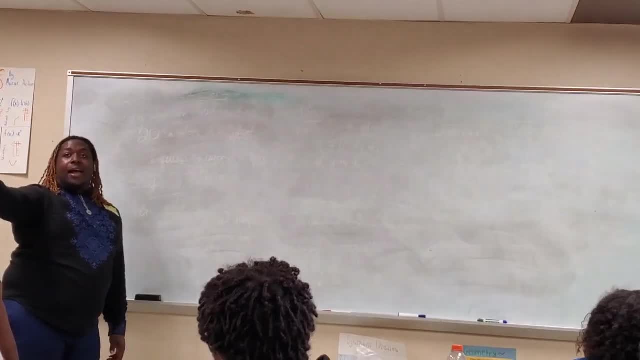 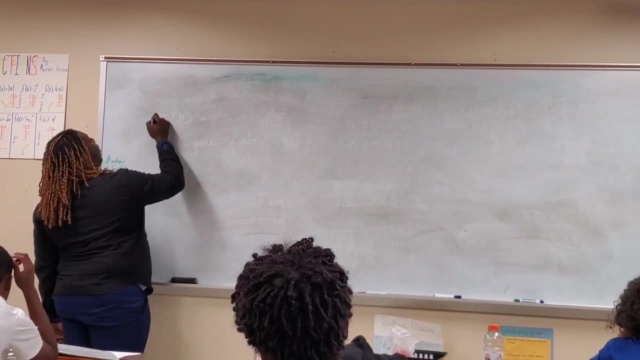 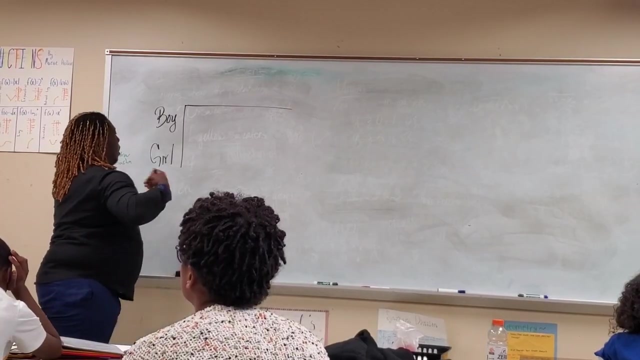 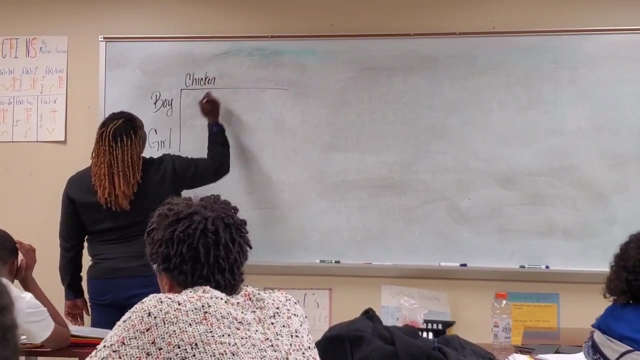 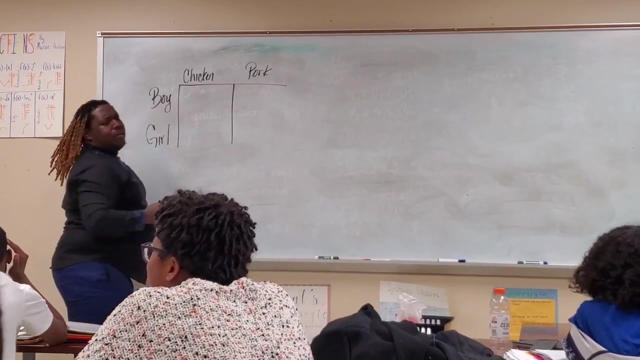 Those in the back have way too many boxes, but those are two-way tables. So let's say, Let's say, In this two-way table at lunch today they were serving chicken, But they were also serving pork, Which probably would never happen in the school. 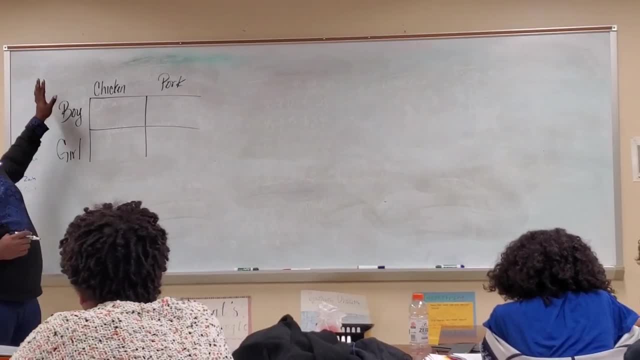 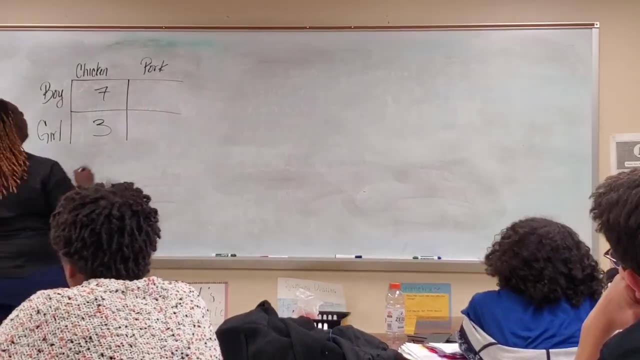 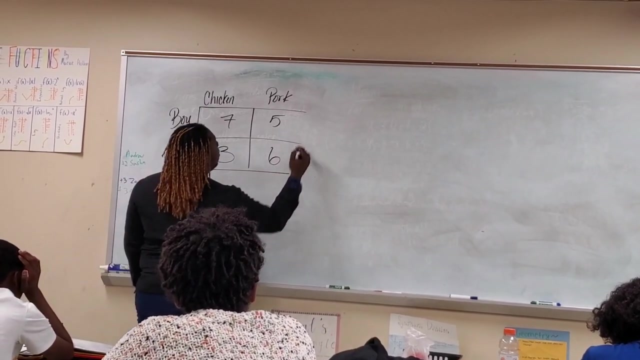 So of all the people in a class, seven boys said they wanted chicken, but three girls said they wanted chicken, And five boys said they wanted pork, But six girls said they wanted pork. So we gotta make sure we have totals. 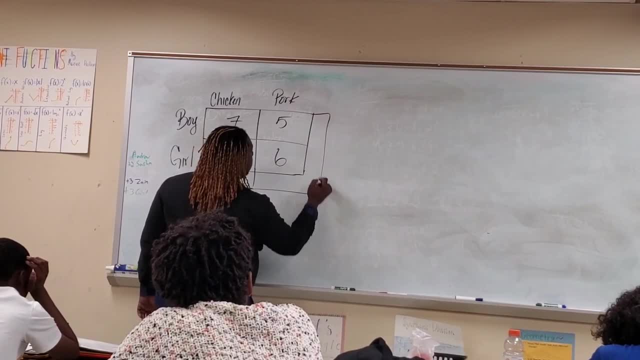 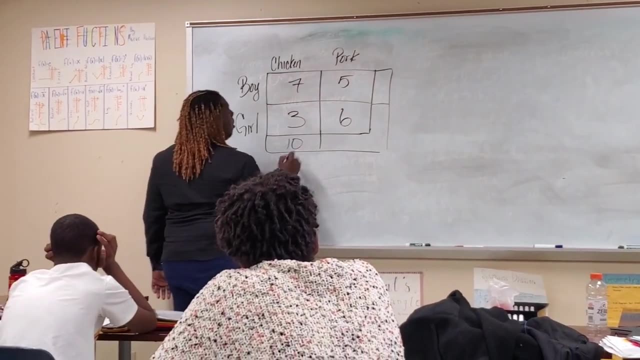 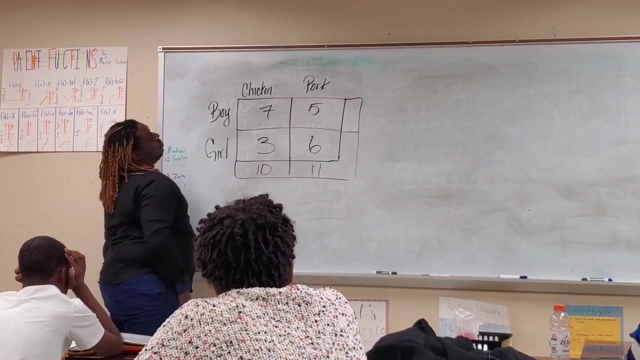 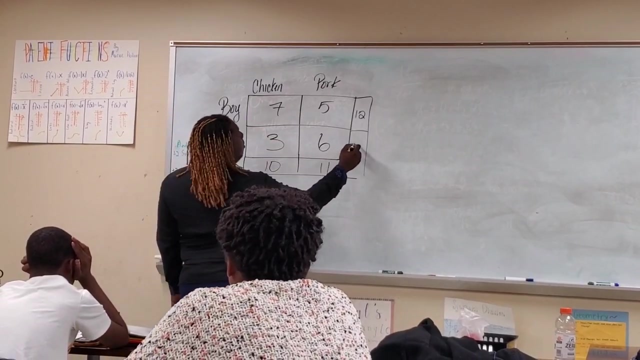 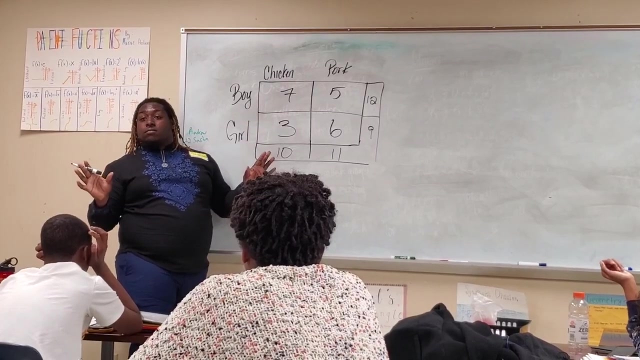 So, in counting the totals, how many people wanted chicken Ten? How many people wanted pork Eleven, Eleven. How many boys ate lunch Twelve? Alright. How many girls ate lunch Nine? Now, I'm not sure how you can get your math wrong. 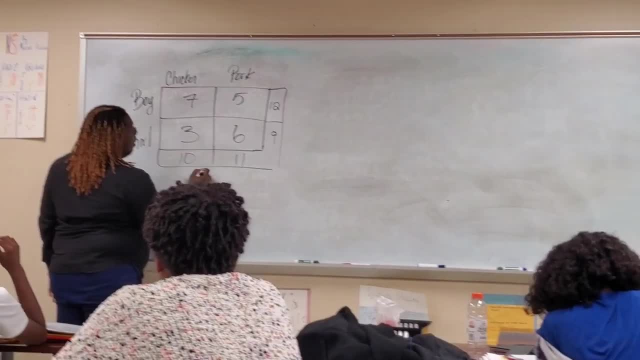 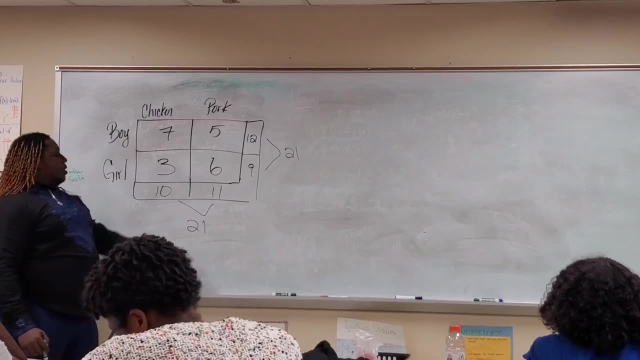 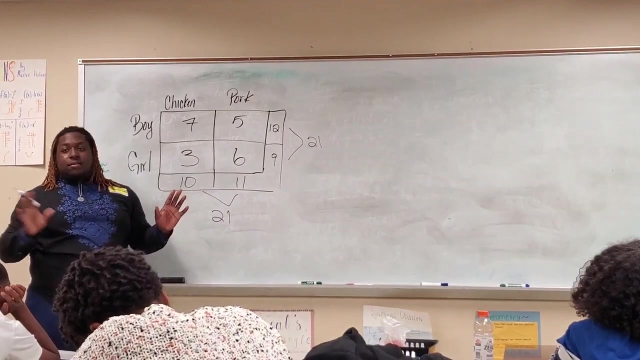 but if you add these numbers up, they give you twenty-one. If you add these numbers up, you get twenty-one. That should always be the case. For some reason, if these numbers aren't the same, then somehow you've done something wrong. 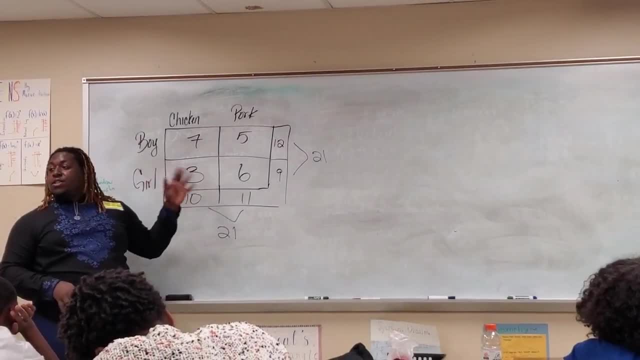 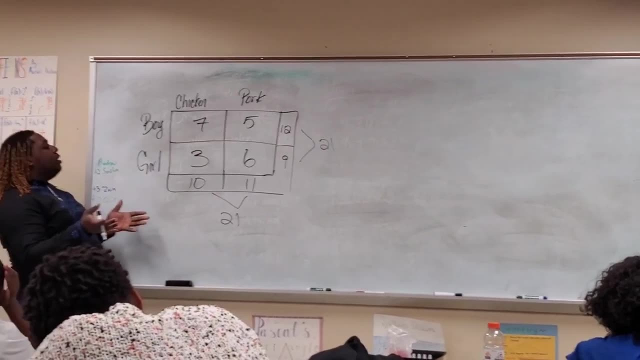 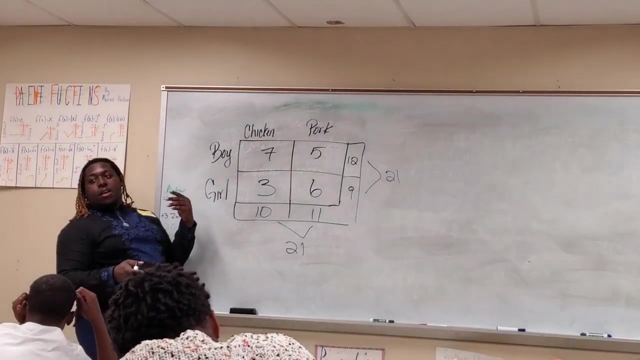 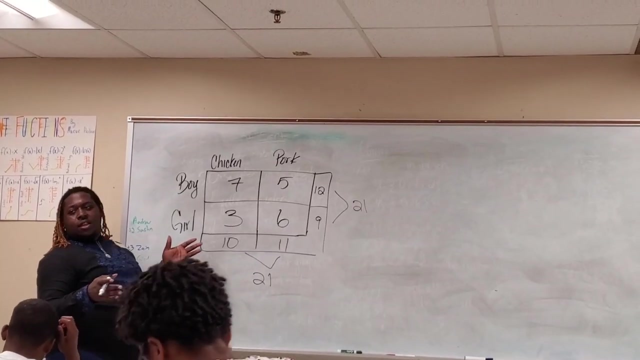 So, looking at probability with a two-way table, Let's say What is the probability that if a student was chosen at random, it would be a boy who wanted chicken for lunch, For lunch, How would we work that? This is somebody I haven't heard yet. 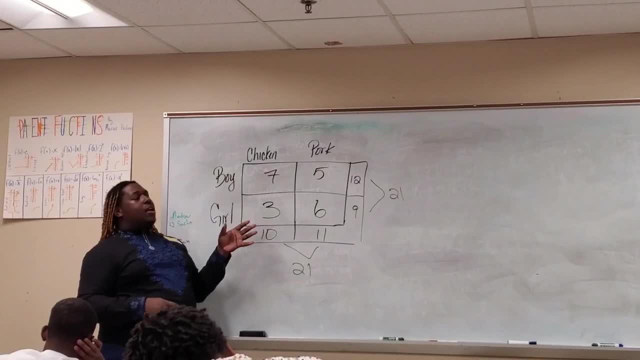 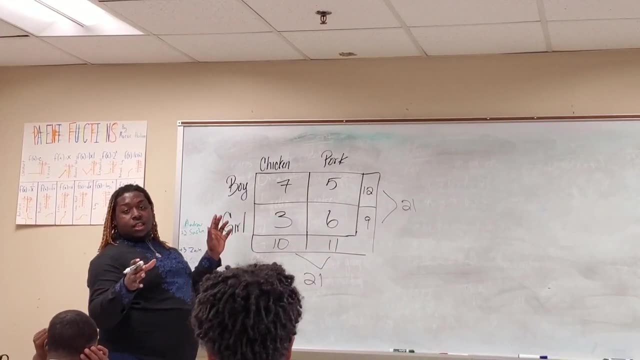 If a random student was chosen, what is the probability that it would be a boy who wanted chicken? How would we work that Seven out of twenty-one? Seven out of twenty-one, Yes. Why would you say seven out of twenty-one? 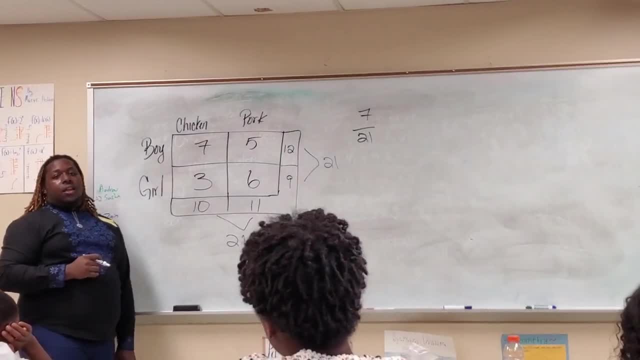 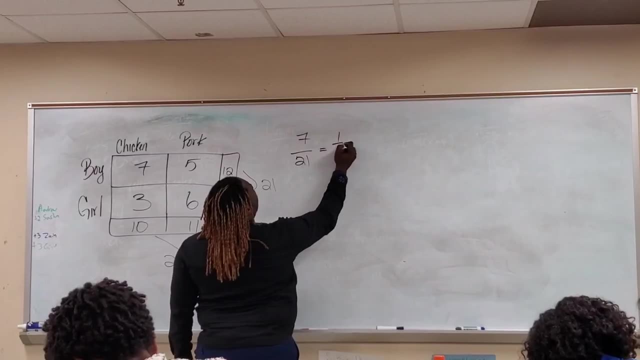 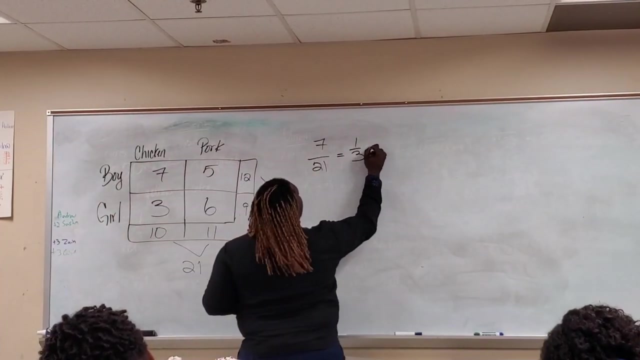 Because there were seven boys who wanted chicken and seven people who wanted pork, Right? So when we simplify that, what is the probability? One-third? One-third? Well, because we know that probability is a number from zero to one. your probability would be .33, or thirty-three percent. 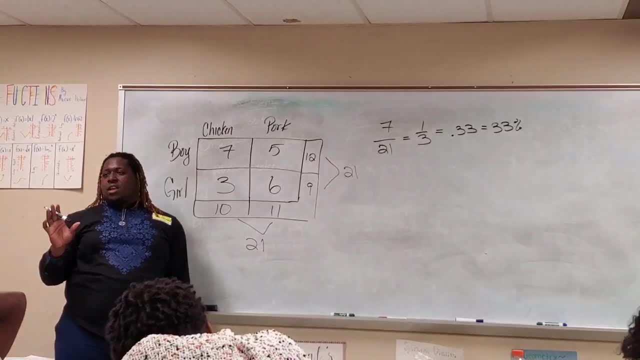 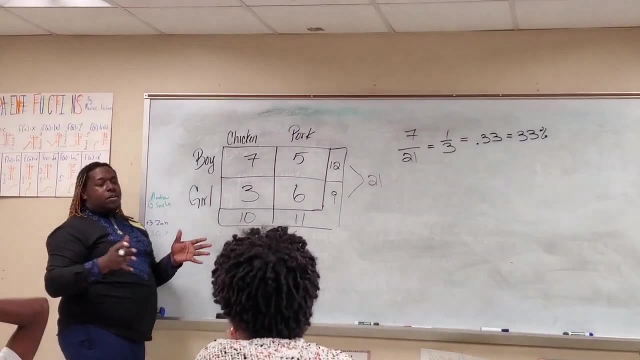 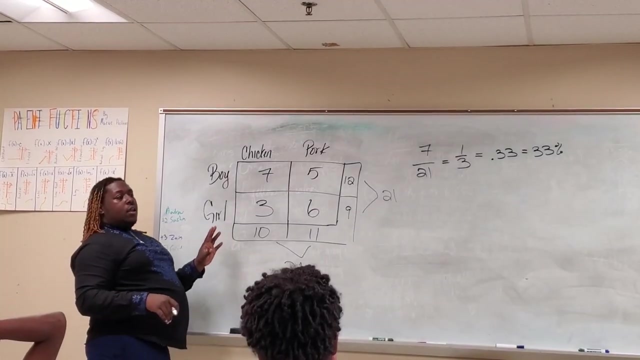 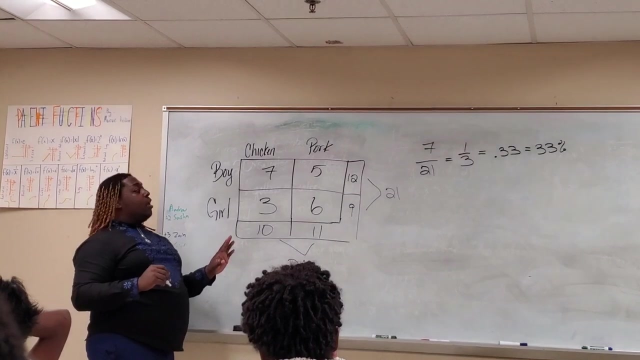 Alright, Are we all on the same page? Okay, So we'll get a little bit more complex. If a student was chosen at random, what is the probability that it would be a girl who wanted pork? If you chose two students, what is the probability that it would be a girl who wanted pork and a boy who wanted chicken? 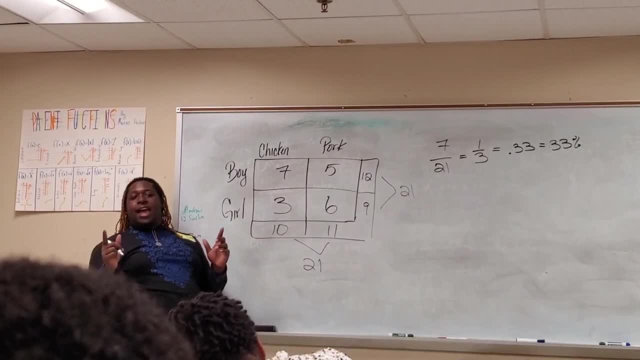 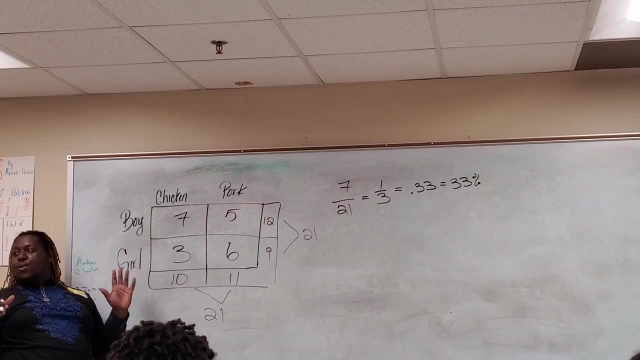 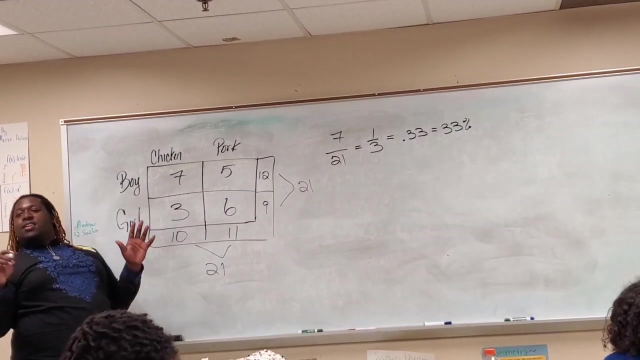 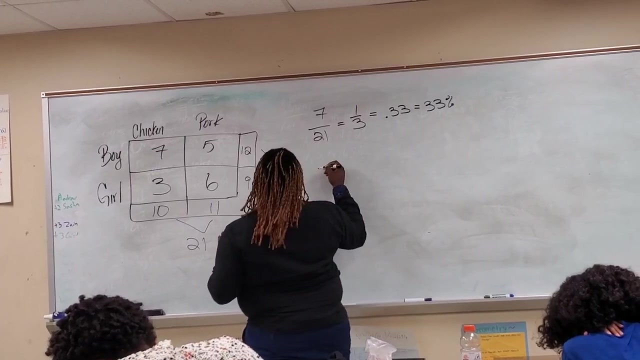 How would we set that up? Somebody- I haven't heard AW, You got it- A girl who wanted pork and a boy who wanted chicken. Close, Not quite. Try using a different operation. So we know that What is the first fraction that we would get? 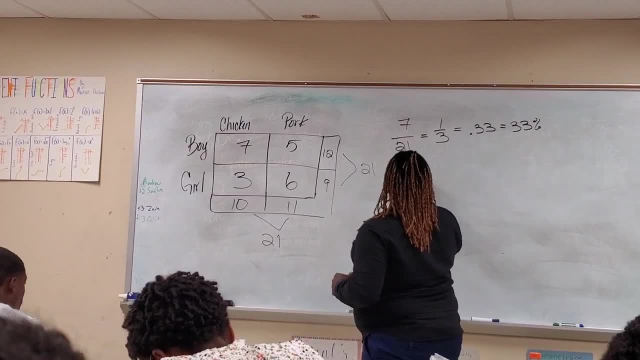 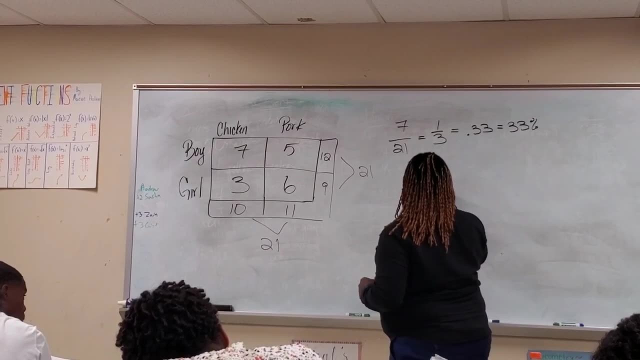 Six over twenty-one. Six over twenty-one, And what's the second fraction that we would get? And what's the second fraction that we would get? Seven over twenty-one? Alright, She said subtraction, But that's not quite the case. 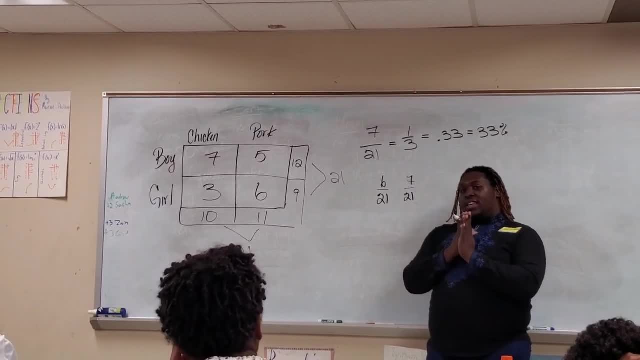 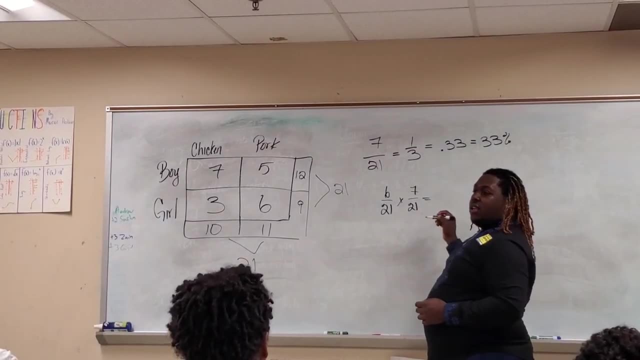 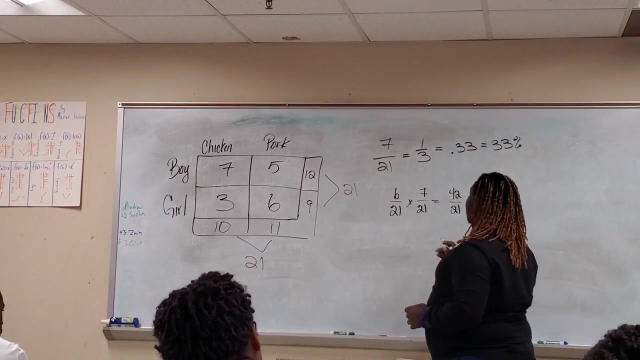 Yes, Yes, It is multiplication. So if you do that, what do you get? Twenty-two over twenty-one, Twenty-two over twenty-one, Twenty-two over twenty-one, Which is larger than one, Which is larger than one, Which is interesting. 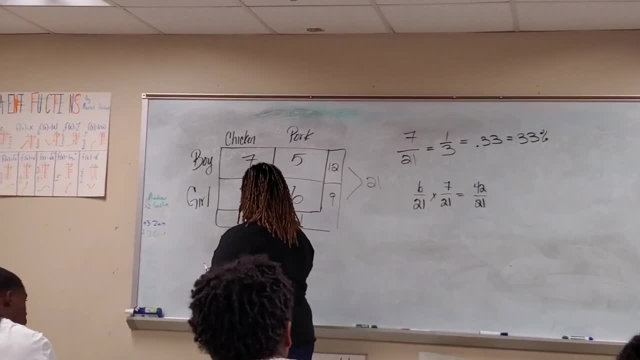 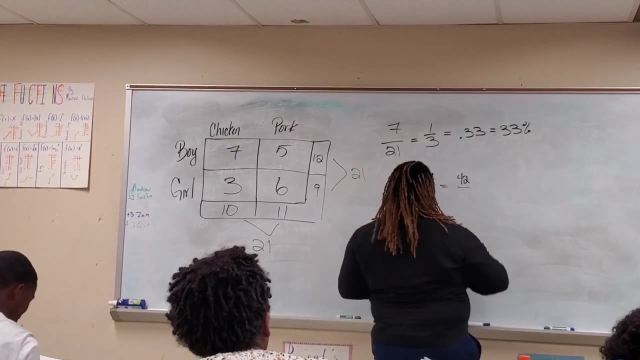 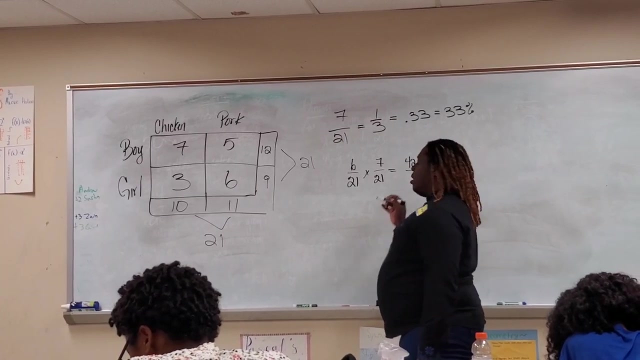 I think it'll work this problem out. The denominators Say it again: Multiply the denominators. That's right. That's why Got to multiply the denominators too. So what would that be? Four hundred forty-one, Four hundred forty-one. 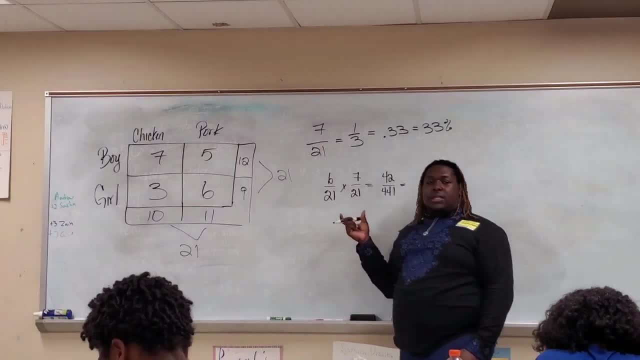 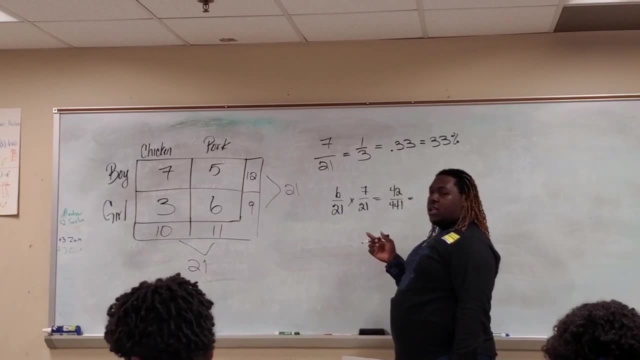 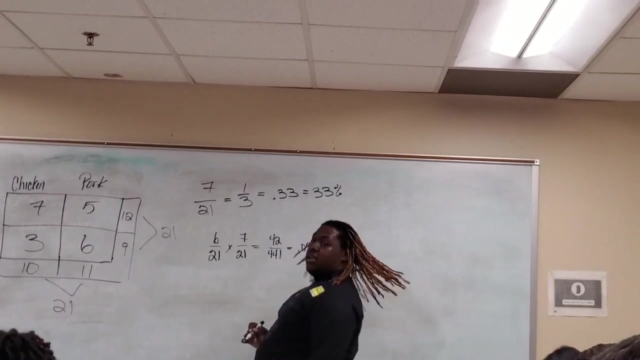 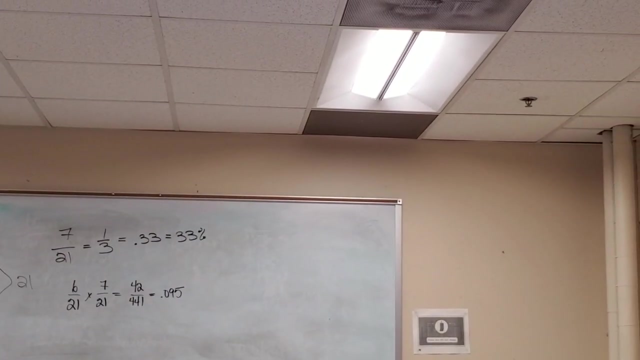 That looks more like it. Alright, so because we need a decimal between zero and one, what would that decimal be? Point zero, nine five. Point zero nine five. Point zero nine five. Alright, Mr Chris. Yes, Would it be the same if you reduced both of those fractions? 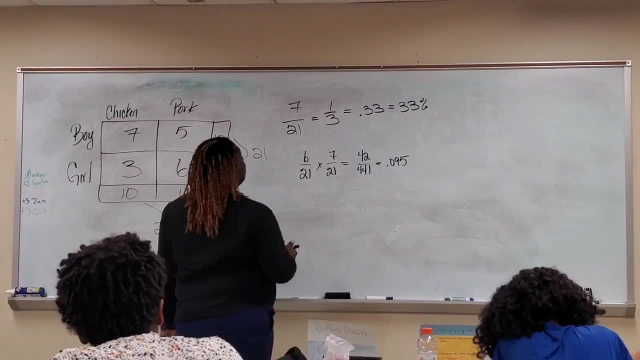 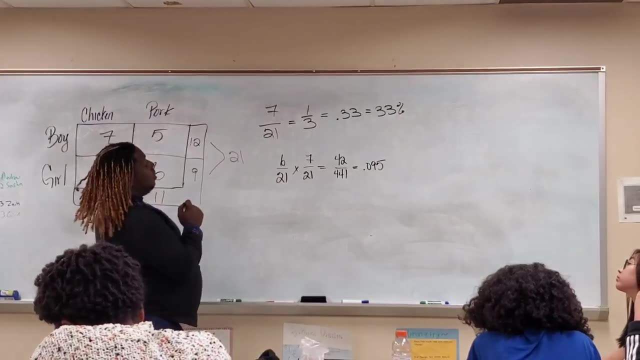 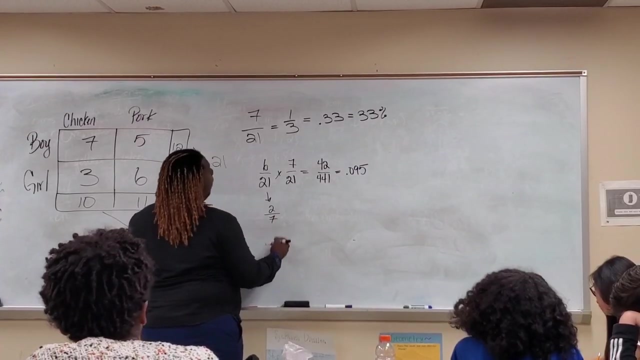 If you reduced the fractions, they should be, So we reduced it. Can we reduce six over twenty-one? Yes, Yes, Divided by three, Divided by three. So what does that give us? Two over seven. And what about this one? 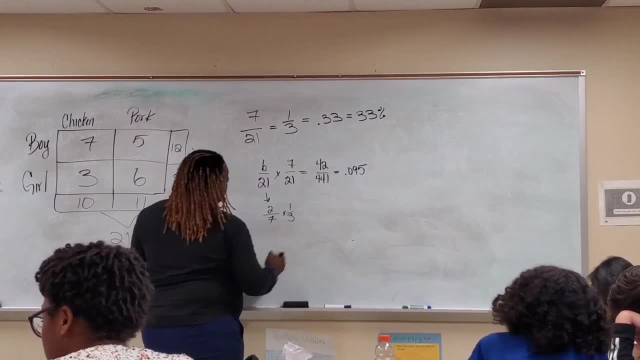 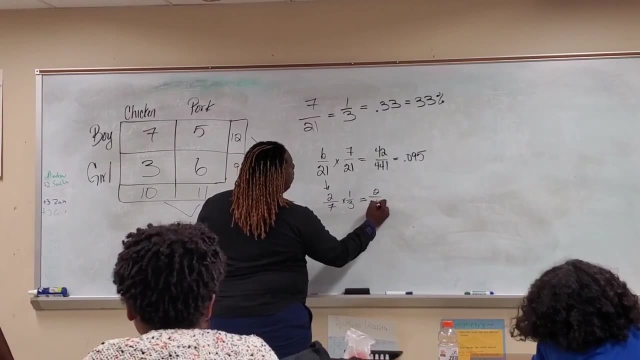 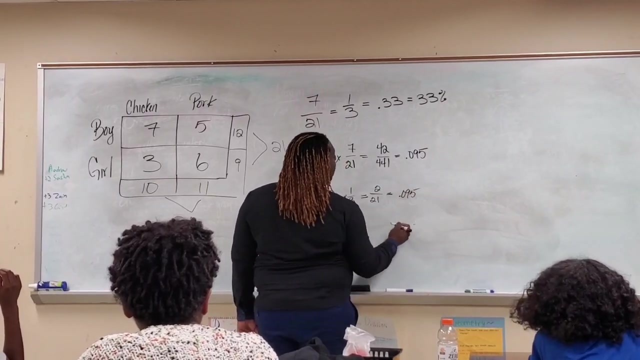 We already said this: one would be one over three. right, Alright. Now if we do that, what do we get? Two over twenty-one. Does that give us the same decimal? Yes, Yes, it does. So it would be point zero nine five. 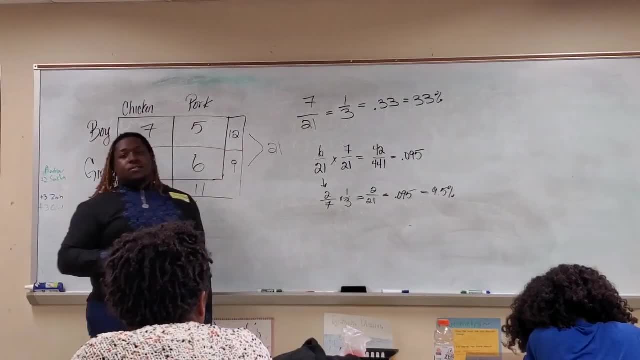 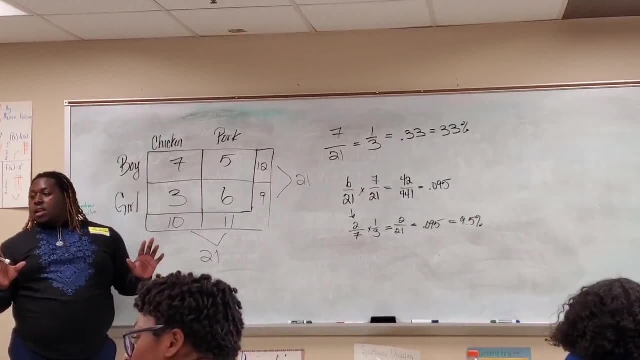 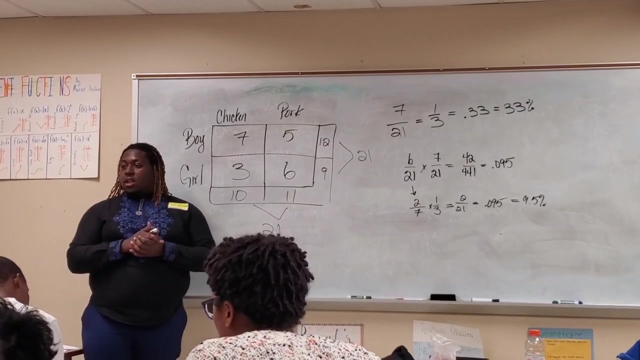 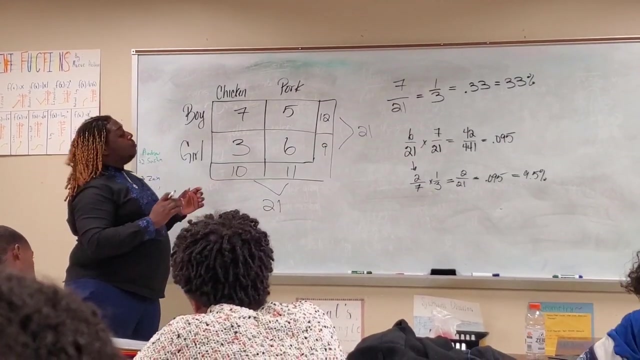 or nine point five percent. Okay, Are we on the same page? Do I need to go over something again With that problem? yes, You said, why didn't we add them? Um, unfortunately, the answer for this is just. that's how probability works.